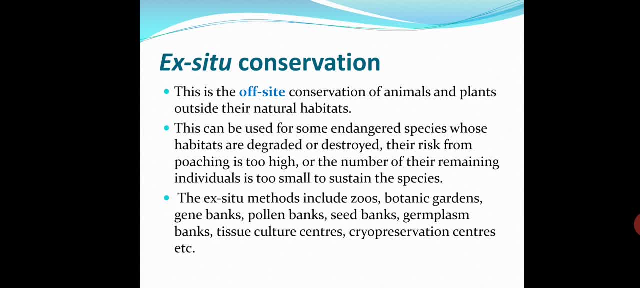 We collect them from where they live and protect them elsewhere. So that is ex-situ, That means off-site. This can be used for some endangered species whose habitats are degraded or destroyed. So in case of tigers, Indian elephants, then lion-tailed macaques. 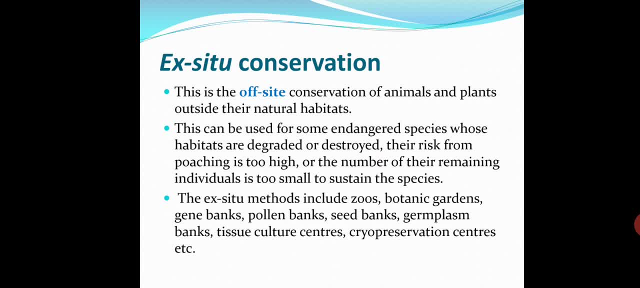 For giving special protection. Suppose we are identifying, by using this red data list, Some organic species, Some organism is under threat, So we can. That threat is due to some habitat destruction Or continuous human anthropogenic activities, So in such cases we can identify these organisms. 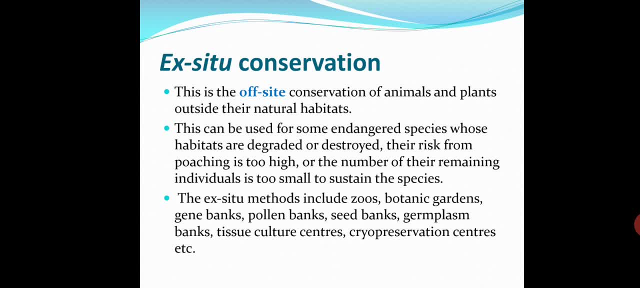 They are under this endangered species or vulnerable species, They can. We can give some separate protective measures. We can provide protective measures outside their habitat, Outside their habitat. Okay, So their risk from poaching is too high Or the number of their remaining individuals is too small to sustain the species. 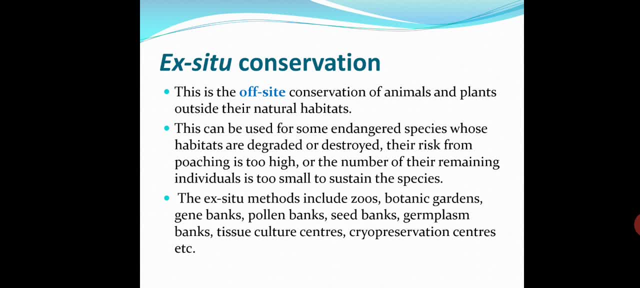 If we identify that there are only a few organisms, we can do this ex-situ conservation. So main methods include: the ex-situ conservation is We can maintain these organisms in zoos Or botanical garden- case of plants, Then gene banks. 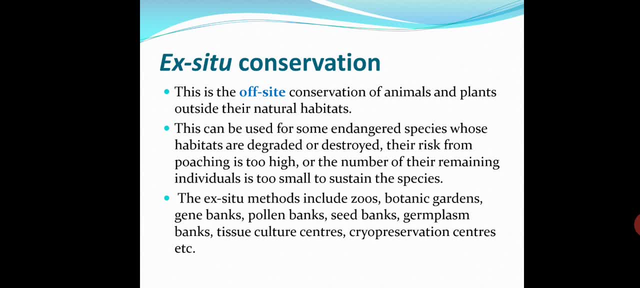 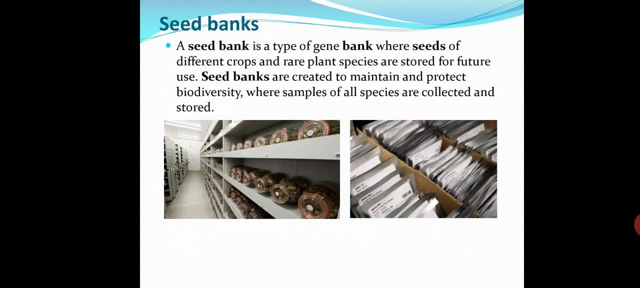 Pollen banks, Seed banks, Germ blossom banks, Tissue culture and cryopreservation centers. So this is how we can keep it Okay. So what is a seed bank? A seed bank is a type of gene bank, So all these are coming under the common head: gene bank. 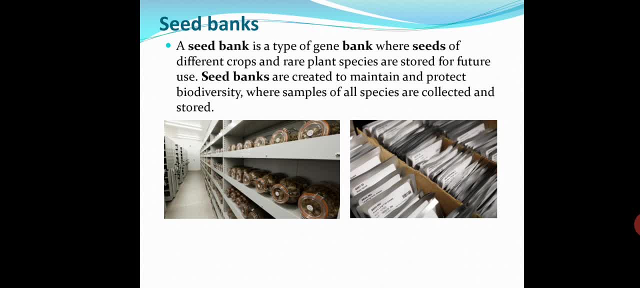 Where seeds of different types, Seeds of different crops or rare plant species are stored for future use. See, I have taken a photograph of this. Seeds are preserved, So we cannot use a lot of chemicals. What is the actual purpose of this storage? 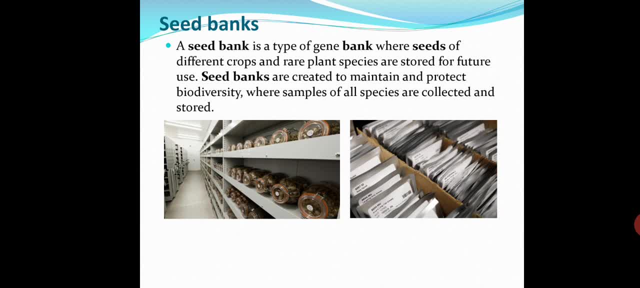 In case that particular plant species is completely destroyed, We can re-generate the plants from these preserved seeds. Okay, So these are old ideas. Now we have seeds of wheat from the graves of pharaohs, So still, it is a viable condition. 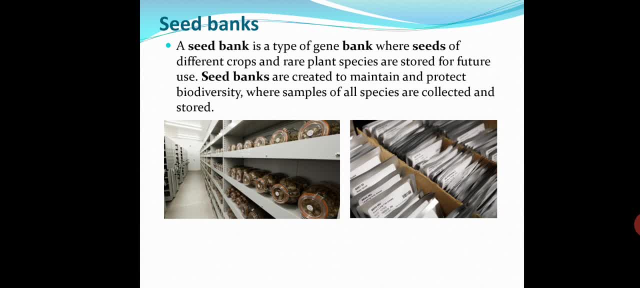 Okay, Even if they are preserved in some way, it is a primitive method. They are used in hygienic conditions And still, some of the seeds and pollens are viable. Okay, So that is what I was saying that day. 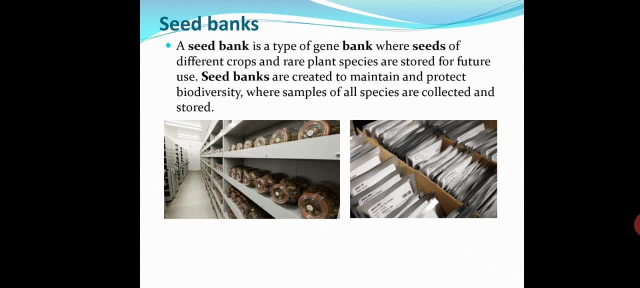 Here we are practicing this mechanism to preserve the germplasm. The original condition of the germplasm can be preserved in the form of seeds. So, as you can see in this, some of the seeds are kept in a bottle. Some of the seeds are kept in a place like a lab where a tissue can be removed. 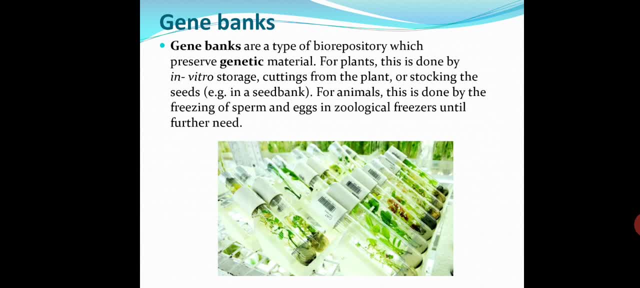 Then the gene bank. The seed bank is a part of the gene bank. Gene banks are a type of biorepository which preserves genetic material And for plants this is done by in vitro storage. In vitro storage- it is not inside the lab. 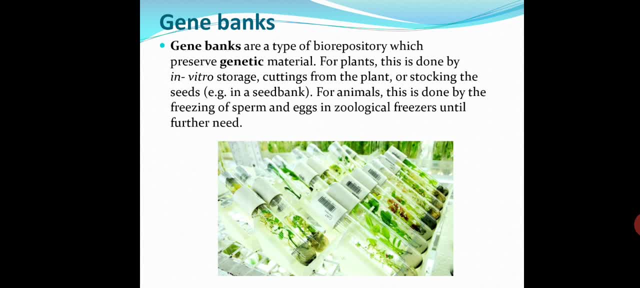 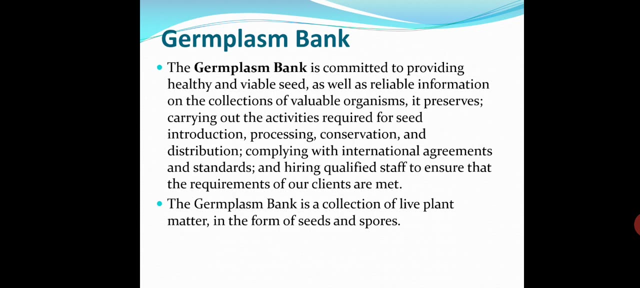 Cuttings from the plant- we can cryopreserve them- Or stocking the seeds For animals. this is done by freezing of sperm and eggs. Okay, This is what we are doing, Then. germplasm bank: The germplasm bank is committed. 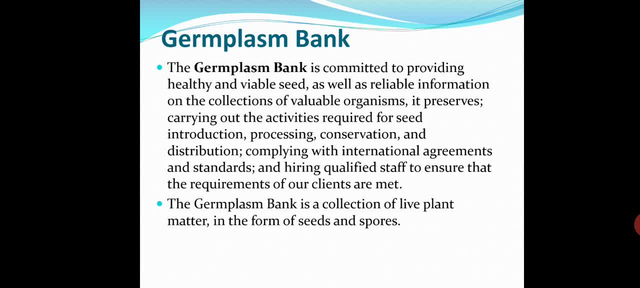 to providing healthy and viable seed, as well as reliable information on the collection of valuable organisms. When we say germplasm, we can modify it a little more. What do we know about germplasm if we grow plants or animals as such protected? 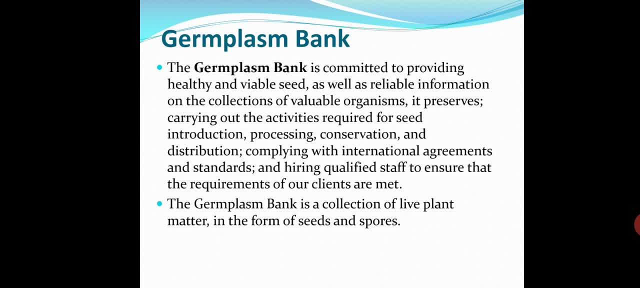 Okay, So the germplasm bank is a collection of live plant matter and also animals, Okay, In the form of seeds and spores or assets. We can grow nuts as seedlings. We can do that. That is what we call germplasm bank. 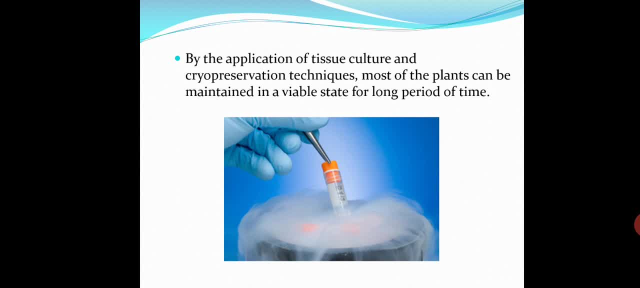 By the application of tissue culture and cryopreservation techniques. we can preserve them in minus degree by using liquid nitrogen, even sperm and eggs. So we can preserve the dead animals, plants or germplasm like this For a long period of time. 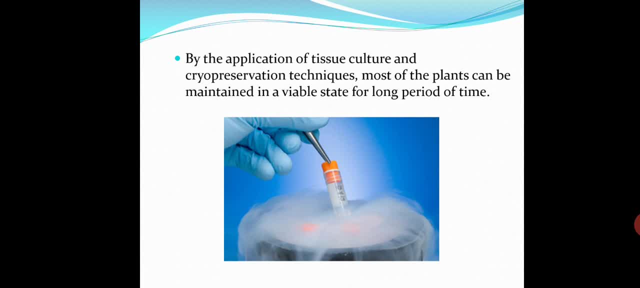 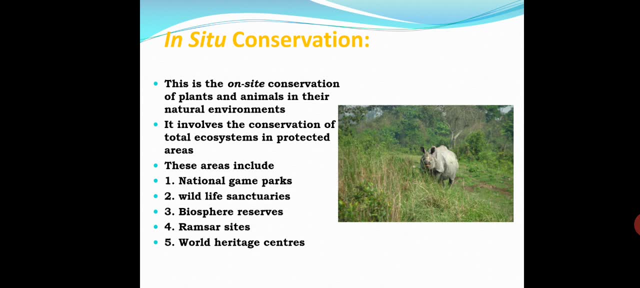 Okay, So it is a type of conservation of biodiversity, Did you understand? Next, we will discuss about this in-situ conservation. Look at the word meaning. This is the on-site conservation. It was off-site Here. this one is in-situ means. 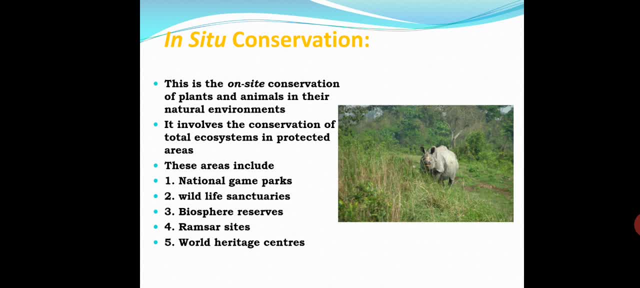 of on-site conservation of plants and animals In the natural environment. It involves the conservation of total ecosystem in protected areas. So when this is in-situ conservation- here is a photo of a rhino of Kasiranga National Park. So when we are protecting- 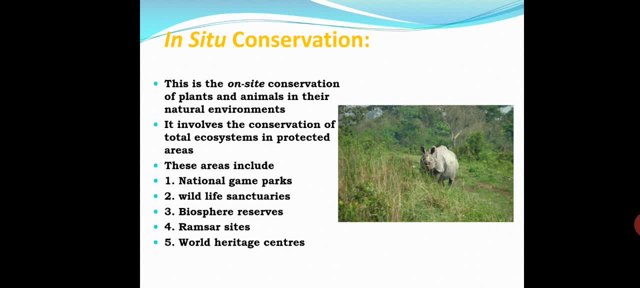 an animal like this, the other organisms in that area- that is last class- we discussed about this- That umbrella species, So we have to remember that too. So this in-situ conservation includes some. we can add in-situ conservation of that is by constructing. 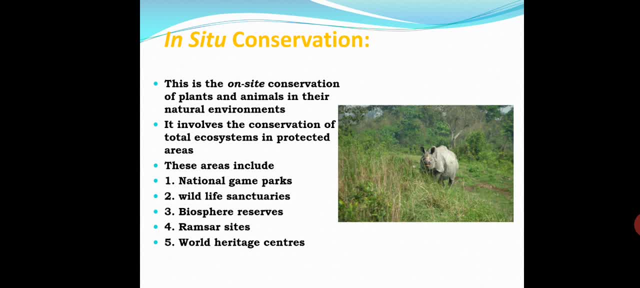 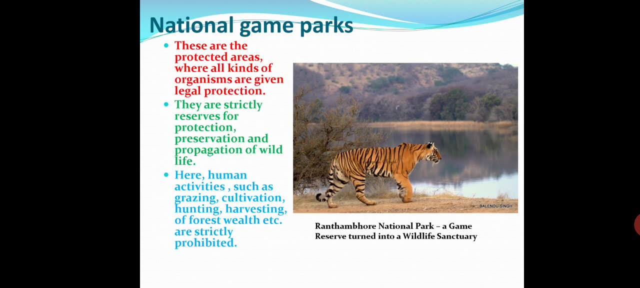 national game parks, wild life sanctuaries, biosphere reserves, Ramsar sites and world heritage centers. Okay, So in this way we can protect this. So let us see each one of them one by one. So, national game parks: 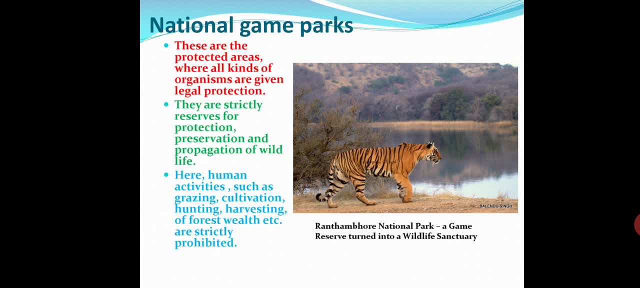 What is this national game park That is? these are the protected areas where all kinds of organisms are given legal protection Under the law. people are protected and hunted inside it. Okay, Generally we can protect this area, Not to mention an animal. 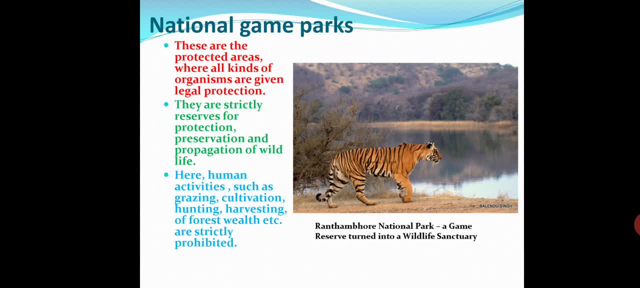 all the organisms in that area. we can protect it. They are strictly reserved for protection, preservation and propagation of wild life. Here, human activities such as grazing, cultivation, hunting, harvesting forest wealth are strictly prohibited. That is the importance. 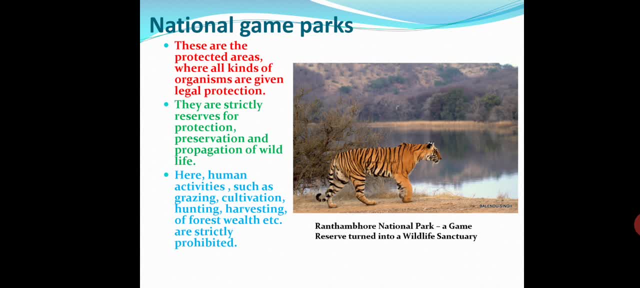 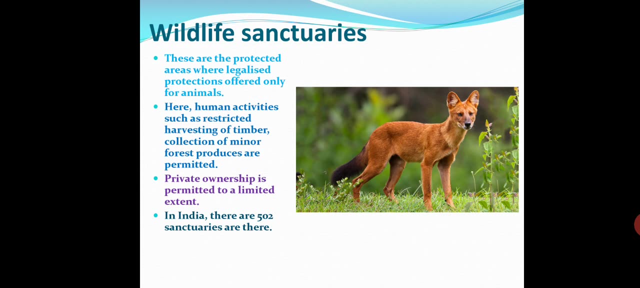 In national parks. this is never allowed, Okay. So I have given an example here. You can see it, Okay. The next one: wild life sanctuary. That is here. these are the protected areas where legalized protections are offered only for animals. 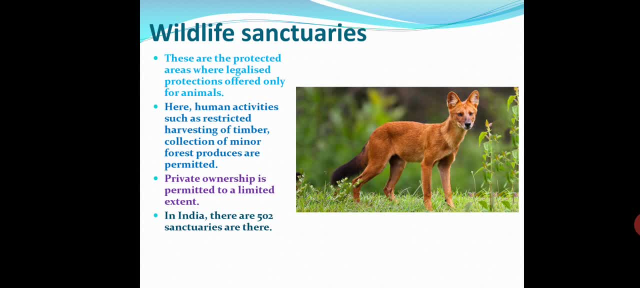 So plants are not included in it. It is only for the protection of animals Here. human activities such as restricted harvesting of timber, Because coming under the wild life sanctuary there is no, only the animals are protected. So what happens there is. 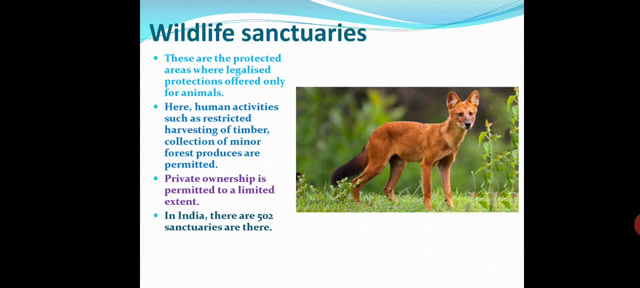 a small number of timber is allowed to be cut down And collection of minor forest producers are permitted. This is also under the forest department. Then private ownership is permitted to a limited extent. Small areas are allowed to be taken into account. 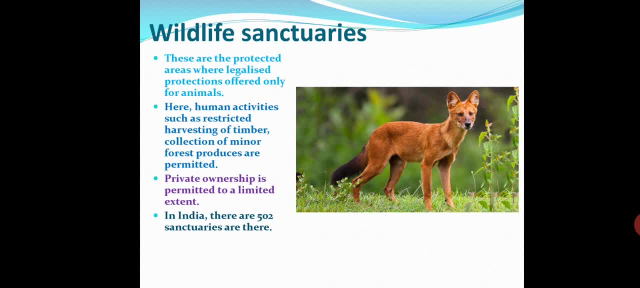 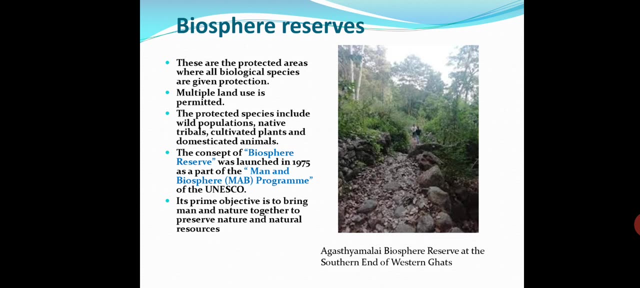 In India there are nearly 502 sanctuaries are there? Okay? So here you can see that this is the difference between the two. Then biosphere reserves: These are the protected areas where all biological species are given protection. 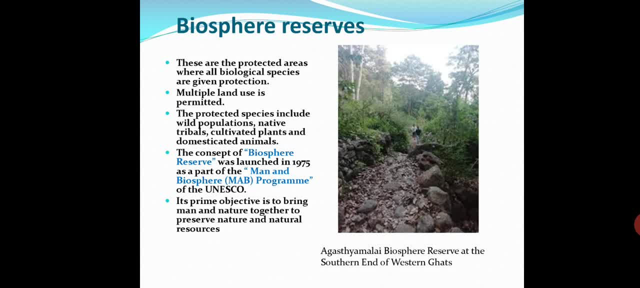 In this, animals and plants are included. Multiple land use is permitted Now. small tribal sectors are seen in between. The protected species include wild populations, native tribals, cultivated plants and domesticated animals, So the same protection is provided to the 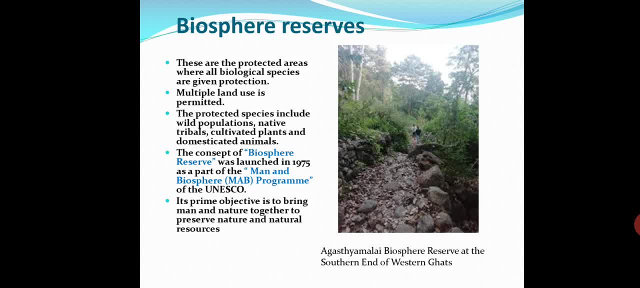 tribes inside this. The concept of biosphere reserve was launched in 1975 as a part of the Man and Biosphere Program. The idea was that humans should not enter into the biosphere reserve, But along with that man and nature should be. 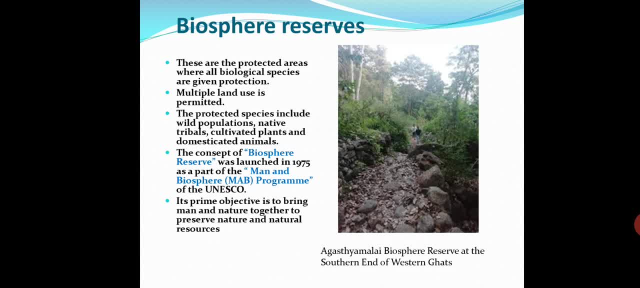 together to preserve nature and natural resources. Here the photograph is the Agastimala Biosphere Reserve. You can see two people walking there. Tourism is allowed only at certain times. The Agastimala is a perfect example of the biosphere. 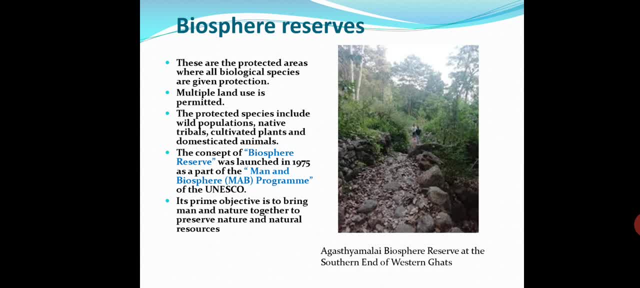 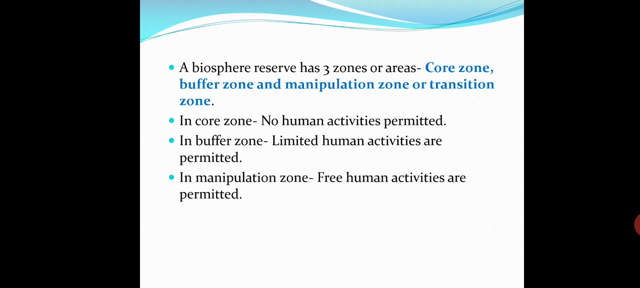 reserve. The Agastimala Biosphere Reserve, is a very important resource for the people living in the Biosphere Reserve. The Agastimala Biosphere Reserve is a very important resource for the people living in the Biosphere Reserve The Agastimala. 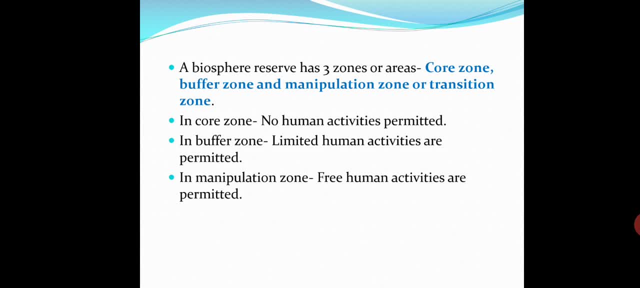 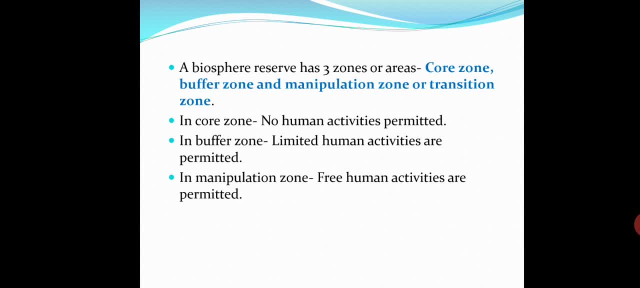 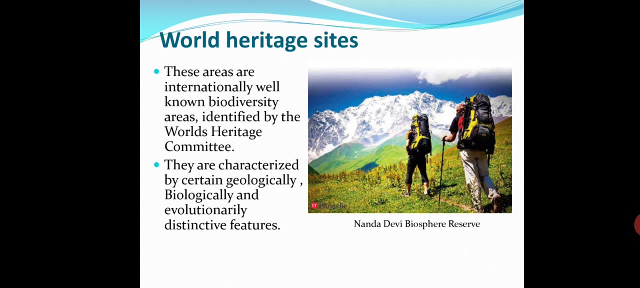 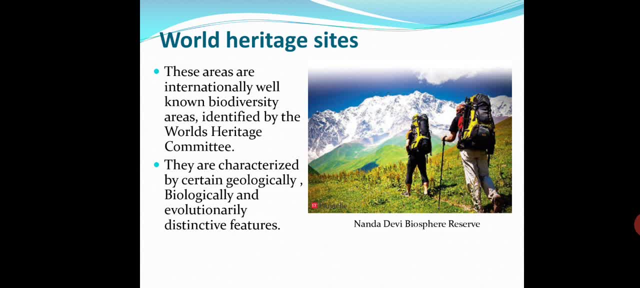 Biosphere Reserve. Agastimala Biosphere Reserve is a very important resource for people living in the Biosphere Reserve. Agastimala Biosphere Reserve is a very important resource for people living in the Biosphere Reserve The Agastimala. 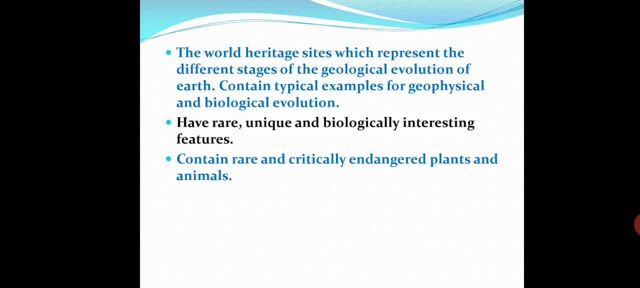 Biosphere Reserve is a very important resource for people living in the Biosphere Reserve. Agastimala Biosphere Reserve is a very important resource for people living in the Biosphere Reserve. Agastimala Biosphere Reserve is a very important resource for. 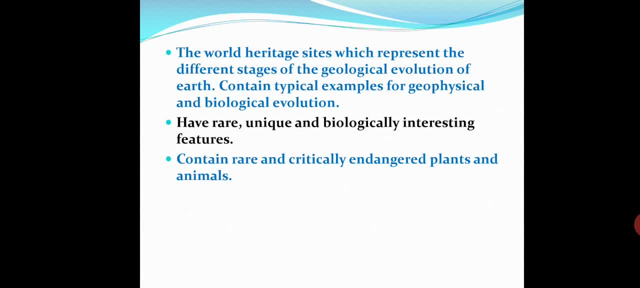 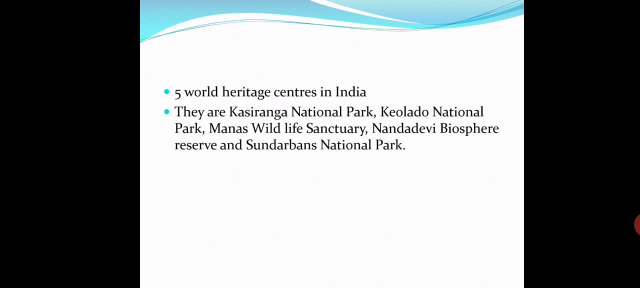 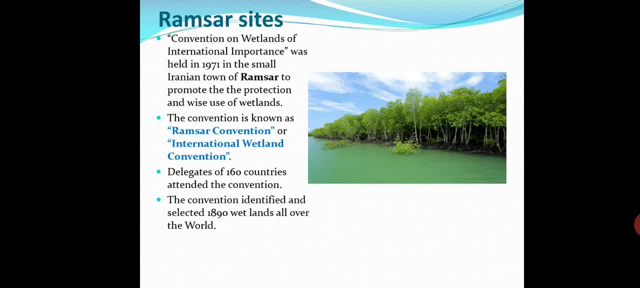 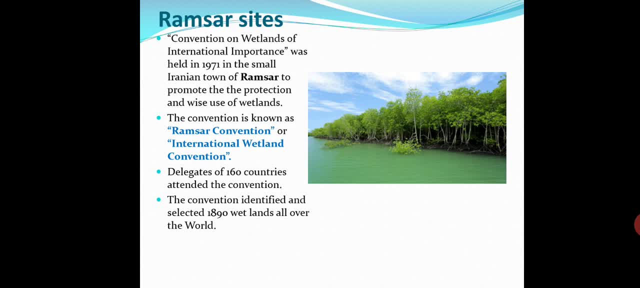 very important resource for people living in the Biosphere Reserve. Agastimala Biosphere Reserve is the most important resource for people living in the Biosphere Reserve. Agastimala Biosphere Reserve is a very important resource for people living in the Biosphere. 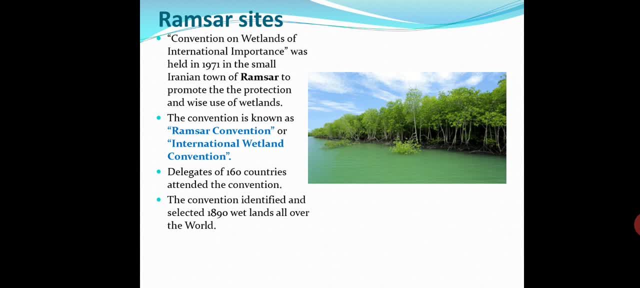 Reserve. The first place where the Ramsar Convention took place was in Iran, So the convention is known as Ramsar Convention or International Wetland Conservation Convention, And not only 160 countries have taken part in it. The convention identified and selected 1890 wetlands all over the world. 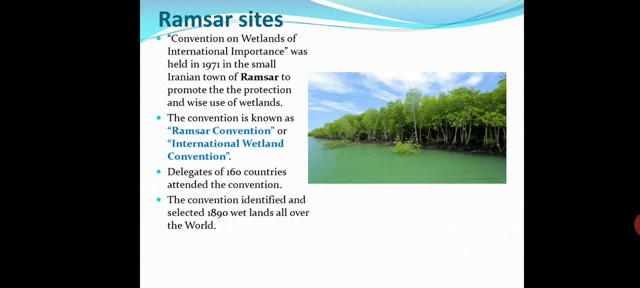 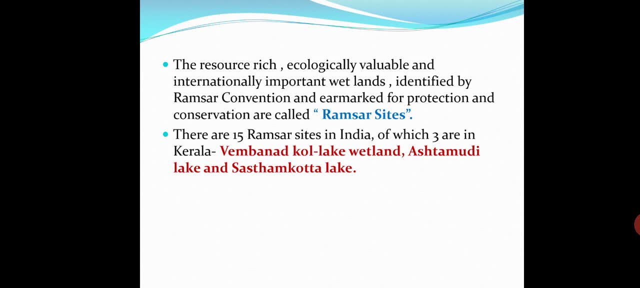 So many areas have been identified since then, And the resource-rich, ecologically valuable and internationally important wetlands identified by Ramsar Convention and earmarked for protection and conservation are called Ramsar sites. So even the local government has identified Ramsar sites. 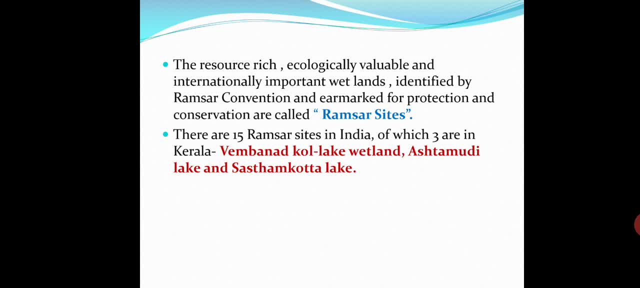 So since then Ramsar site usage has increased. If a wetland is in need of protection, then the government will identify that wetland And the site is earmarked as Ramsar site, Then it is not the protection of the site. 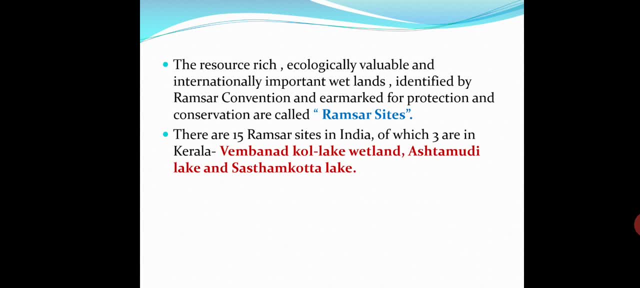 We are not talking about the protection of the wetlands. These are the regulations decided by the convention. There are 15 Ramsar sites all over India, Of which 3 are in Kerala, That is, Vembanadu Coal Lake. 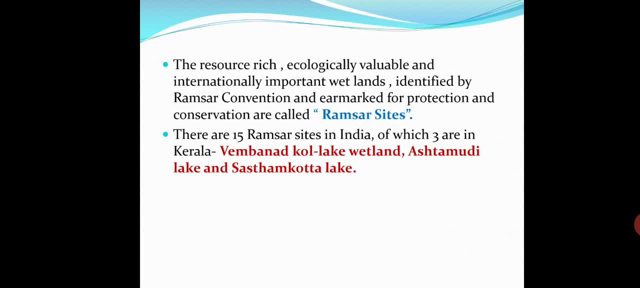 Coal Lake means Salt Lake, Coal Lake, Wetland, Ashtamudi Lake and Shastankota Lake. So in Kerala, if you ask about the four marks, we have to add one or two sentences, That is, first you have to write the importance of wetlands. 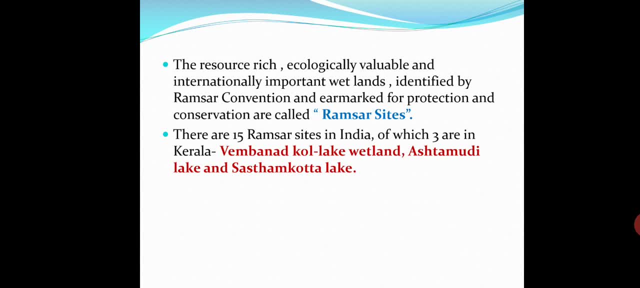 Then about a few lines about the Ramsar Convention And what is the meaning of Ramsar site And these three in Kerala. These are Vembanadu Coal Lake Wetland system, That is, we know, Vembanadu, which is in this area. 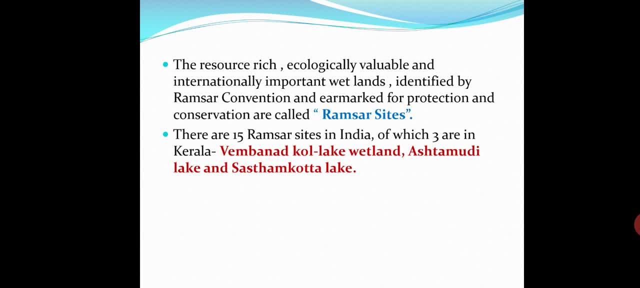 And it is the largest Exurian wetland system in Kerala, With an area of 1500 sq km, And it was included in the list of Ramsar sites in 2002. In 2002.. It was added in 2002.. 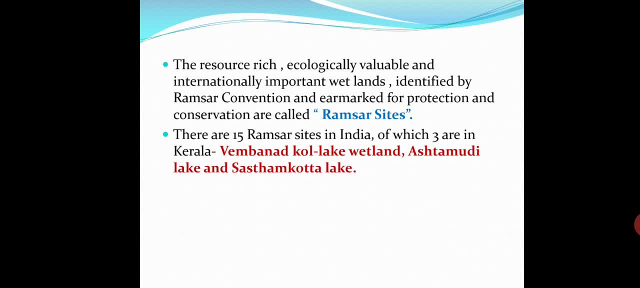 The Vembanadu wetland system is fed by 10 rivers. How many rivers come to that lake? 10 rivers come to that lake, Which many of are from Western Ghats And flow down to Arabian Sea, And that opens the Vembanadu lake to Arabian Sea. 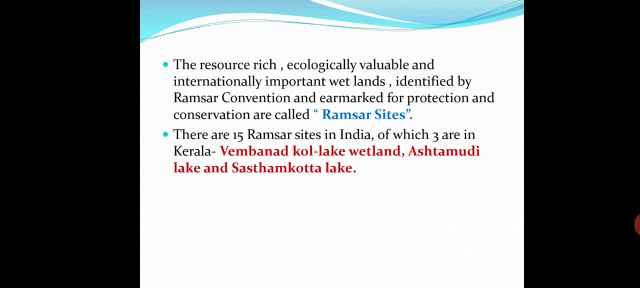 And the system is remarkable for its rich clumps resource. Also, it supports a large population of waterfowls, The most vulnerable sport-billed pelican Migratory birds come to these species every year. That is why Vembanadu Coal Lake is considered as 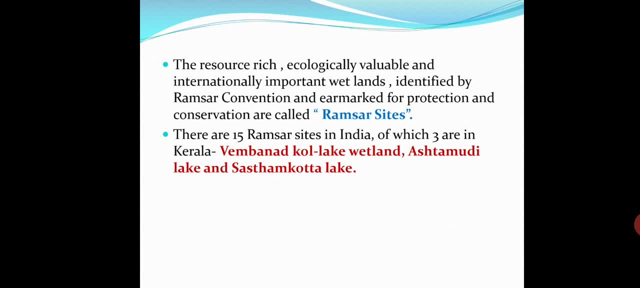 the Ramsar site, Then in Vembanadu wetland system. it was facing severe threats of massive degradation and destruction Due to many of the agriculture. waste is deposited there From coconut plantations then some factories. they are taking affluence. 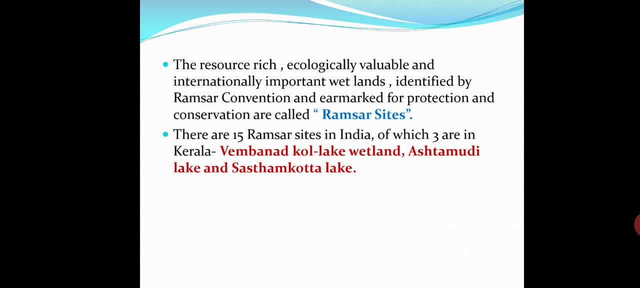 Then coconut husk rutting, So it is making severe threat to the flora and fauna of Vembanadu Coal wetland system. In 2002, this was identified as a Ramsar site. Now it is considered as a criminal offence. 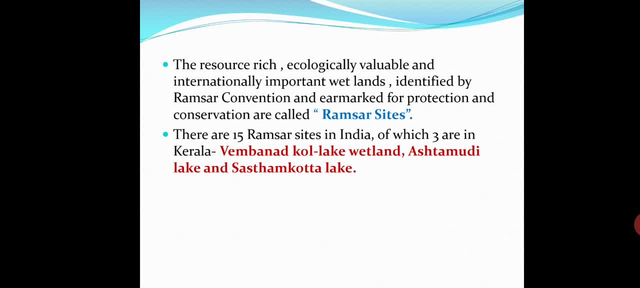 And next is Ashtamudi Lake. So it is the second largest and also the deepest texturian wetland ecosystem in Kerala And it is also included in Ramsar list in 2002.. And it is situated where It is situated: in Kollam district. 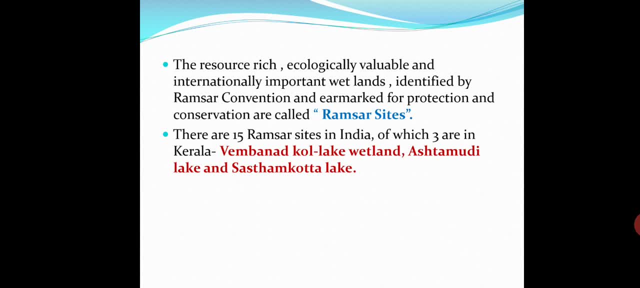 It has a single outlet at Neendakara. It is the only outlet that comes to the sea from Neendakara, And the lake is fed by Kallada river originating from Western Ghats. The other thing is that it is big. 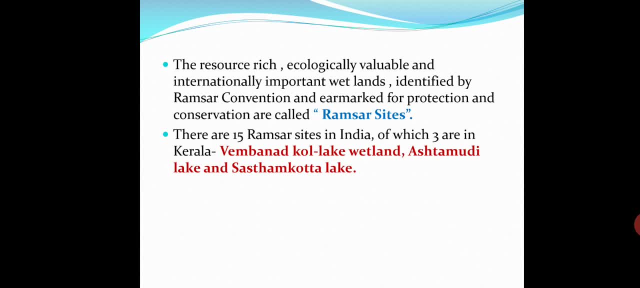 It has 10 rivers that comes to the river Here. Ashtamudi has a single river, That is Kallada river. Then Ashtamudi Lake is under serious threat. It is the same Due to the affluence and paper mills. 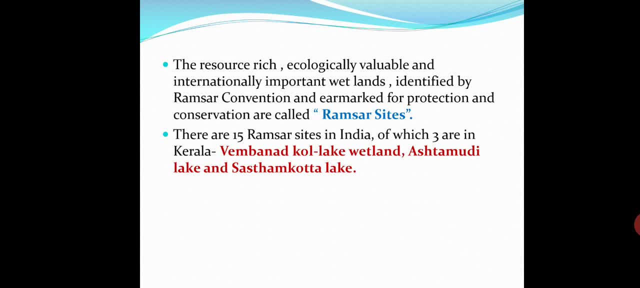 aluminium and ceramic industries are nearby, Titanium factory is nearby And oil spills from fishing boats are coming, Coconut husk rooting- All these are happening inside this, Then Ccgm Travancoricum- It is an endangered plant species. This is Ccgm Travancoricum. 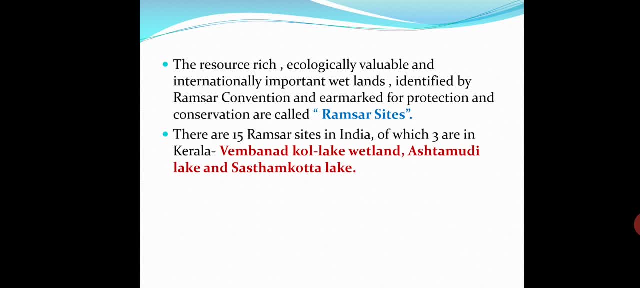 More than 40 species of mangrove plants are in this. So Ccgm Travancoricum is not a mangrove, but it is a mangrove associate. Okay, Next third one, that is, Shastankotta Lake. 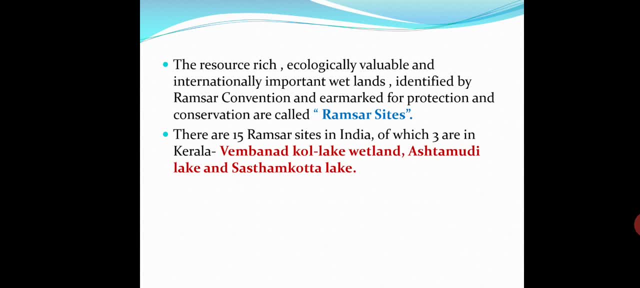 It is the largest freshwater lake. That is my specialty. It is the largest freshwater lake, Having no access to sea. It is never connected to the sea. That is why it is maintaining its freshwater And it is located in Kollam district. 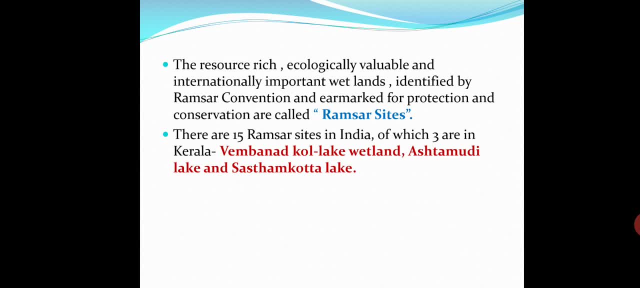 It was also included in Ramsar in 2002.. And there is no river connection. It is like a pond. It is like the largest pond, Even though it is coming under a lake condition. it is not connected to any river or sea. 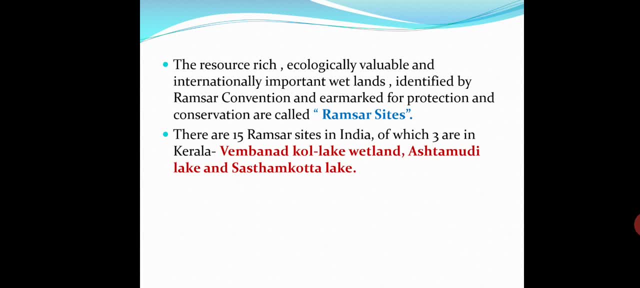 But it is filled by underground sprouts. That is my specialty. It is like a general lake. It is filled with water from underground. I am going to show you how I fill this. See the speciality of Shastankotta Lake.